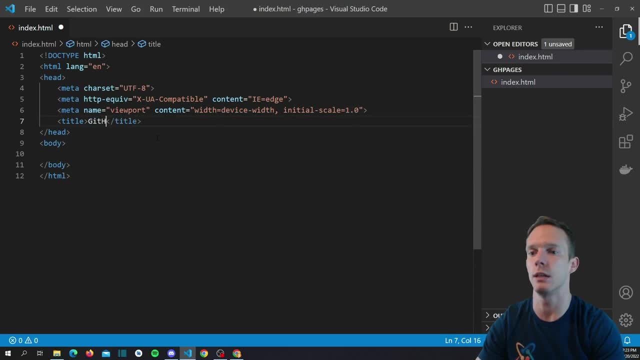 and we can go ahead and stub that out real quick and we'll just call this github pages and in our body let's go ahead and do an h1. we'll say hello world- pretty typical, uh. let's do a little paragraph and we'll say: my name is matt. 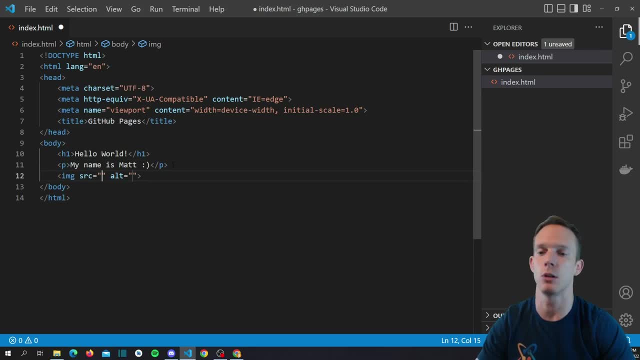 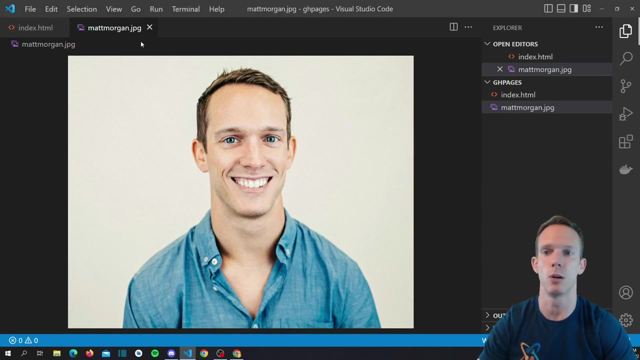 little smiley face, why not? and then we'll put an image underneath it. so let's try to find an image real quick. um, let's go ahead. let me see i have an image of me somewhere on here. all right, matt morganjpg. perfect, hey, look at that guy. um, all right, so let's close that. and if i actually so, 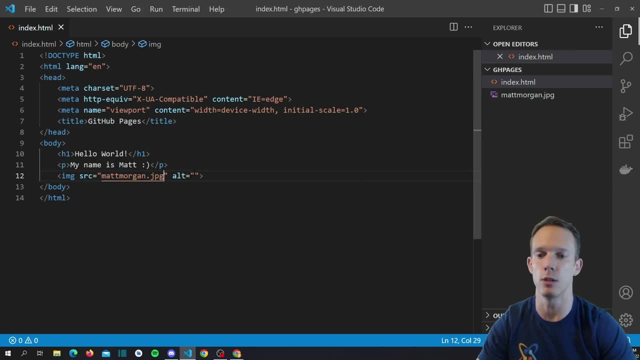 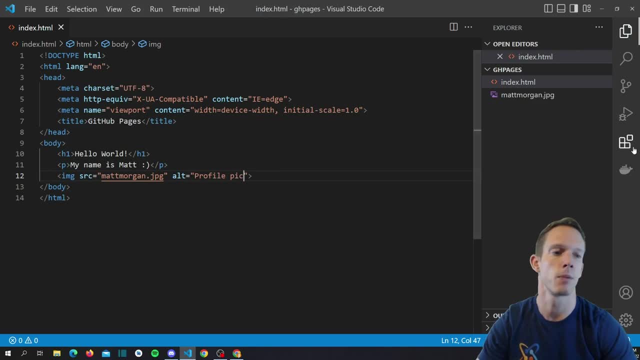 you know, do an alternate. you know profile pic text, um, but the way github pages works it actually follows a jekyll schema and so if you actually try to go to this, it'll try to go to an actual route. so, um, or a web page, so it'll be like slash matt morgan dot jpeg and i don't think it's a. 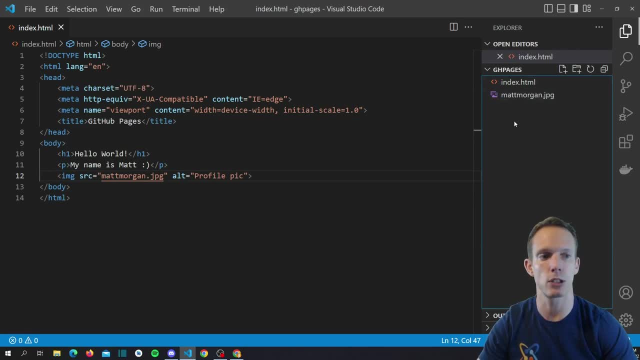 web page, which is ridiculous. but either way, we actually have to do a little bit of uh maneuvering here, and so we'll add a folder and we'll call it assets and then, um, so it needs to be an, it needs to be a folder called assets and then, by default, most of the time it's kind of a. 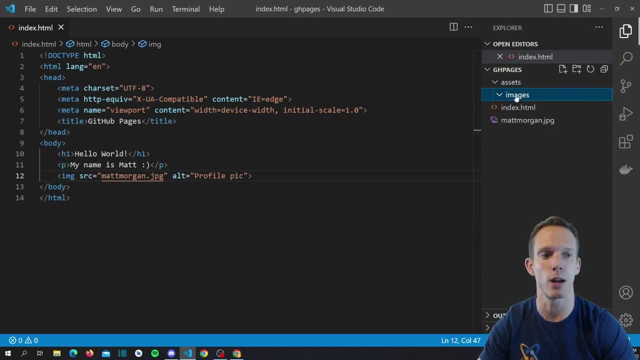 standardization to put an images folder inside assets. but i don't think you actually need this folder, so you could just put it directly in the assets folder. but we'll put an images folder just because usually you'll have more assets than just images and so it's pretty nice just to always have. 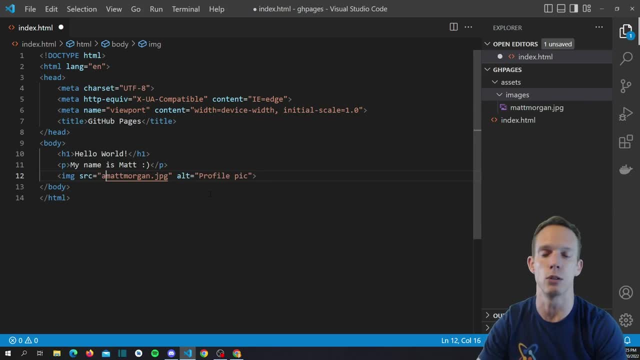 that images folder in there. and so now what we'll actually do is we'll put assets slash images like that- oh, slash map more- in a jpeg, all right. and then what we can do is we'll go ahead and link a css file too. so linkcss, stylecss, and i believe you can actually put the stylecss file in the. 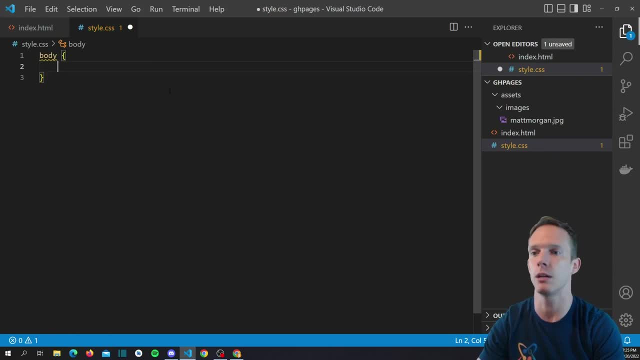 root, which is a little strange, but again, don't ask me why it's the jekyll the jekyll way. if it doesn't, we may have to move it into an assets folder as well, but i don't believe you need it for css, so body will. 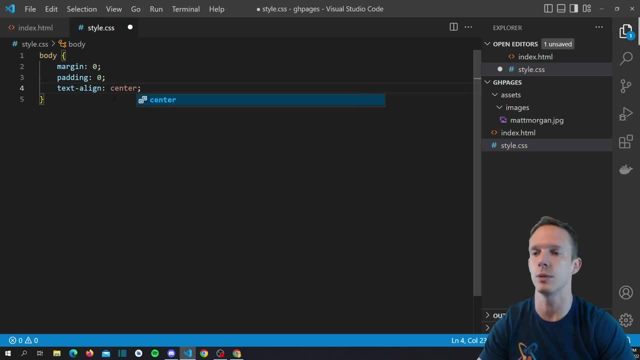 put margin and padding zero and then we'll just text align everything center. i mean, we're not, we're not trying to style this thing to look great, uh. but we'll say h1 and we'll say: you know, padding top four m's, and then let's see the paragraph. it probably comes with default margin, but let's just. 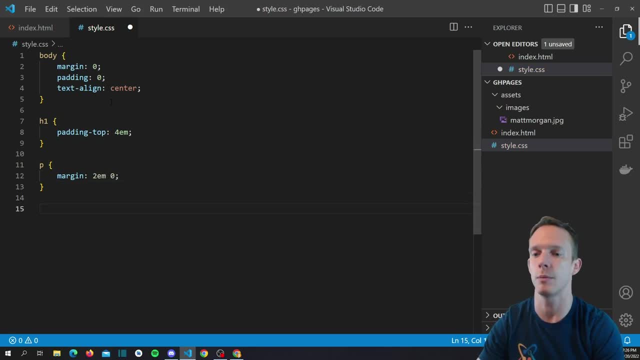 set it um: two m's top and bottom, zero m's on the left and the right, and then our image. let's just say: uh with, let's make it, let's make it big, let's do 40 m's, max width, 90, just so that it looks good on mobile too. we're styling for mobile and desktop. 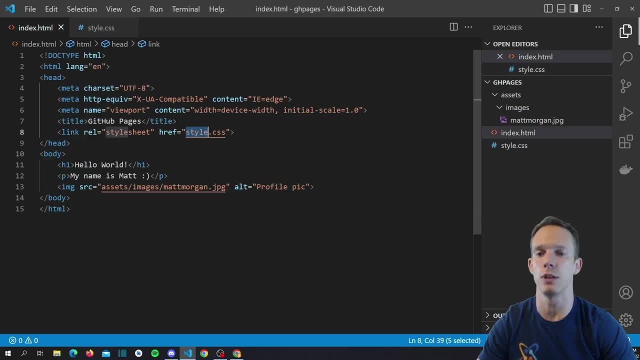 all right, so pretty basic styles. uh, hopefully that actually gets applied. but what we're actually going to do now is we're going to show you actually how to get this thing deployed. so imagine this is actually just a regular project and open up github. i've already created this. 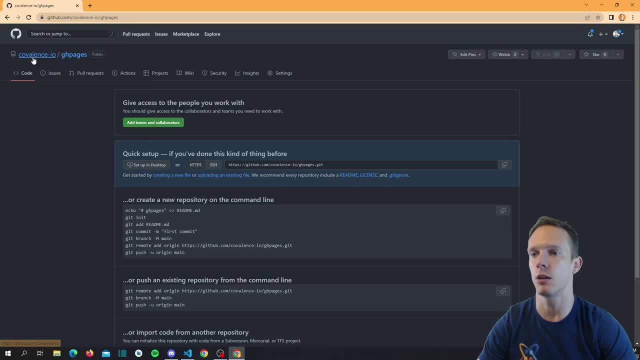 repository called gh pages. this is in our actual organization, but it wouldn't matter if it was your. uh. github actually allows you to do unlimited webs or github pages for projects. now, it just has a separate url and so, uh, it's specified by the repository. they allow one github repo. 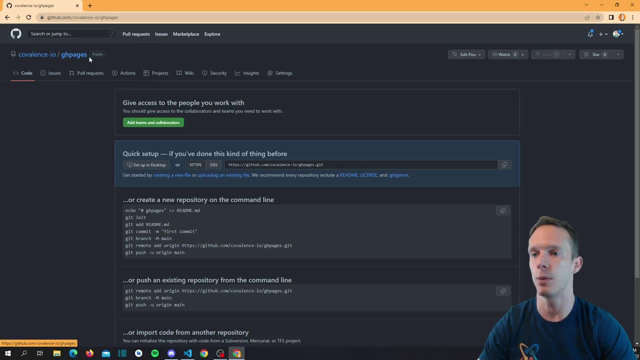 per person or per organization, but then unlimited per project, and so, if you want like this, there's, you can actually have a standard website for just your organization that has, you know, a better looking url, and you can actually add custom urls, i think now too. so it's getting pretty robust and 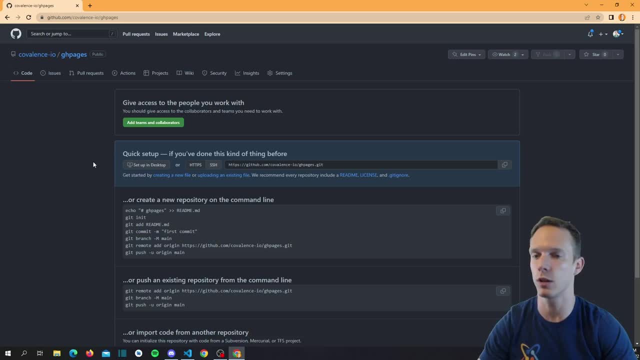 if you want to do something with a build process, you actually could, so you could deploy. i believe you can actually deploy something like a next js project now, but i'm not certain about that. if you know for sure, drop it in the comments below. i'd love to actually 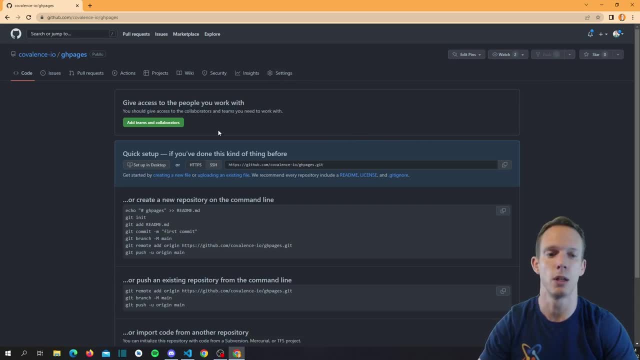 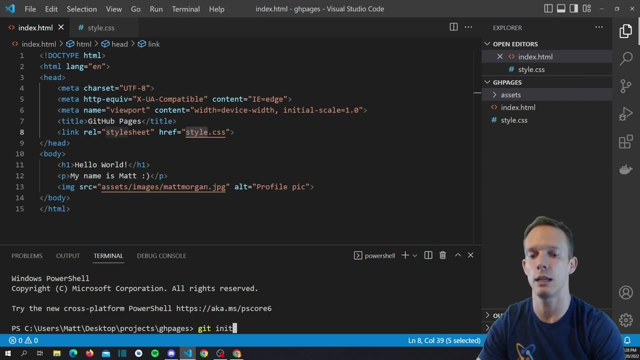 do a future video on that, because i'm sure it's possible. but again, it used to not be possible. but i think now you can do it with github actions. but let's go ahead and get this repo ready. so we're going to open up terminal and we're going to get a knit it and then we're going to get add. 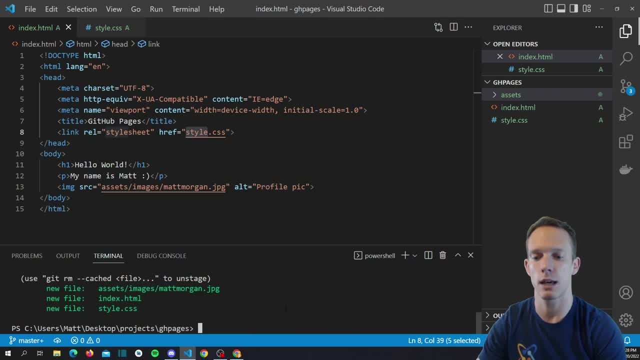 everything. so get a get add dash a get status. just a look, all right, so we'll get commit um initial commit, all right, so we're in there. um then we can get, we can make the branch main, and they've been pushing that for a while. so if you want, you know, get on the main branch, or 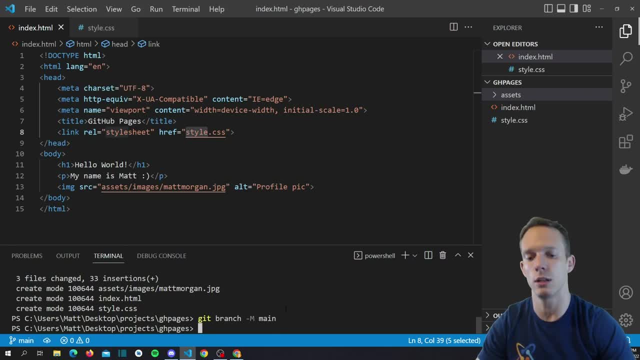 and, uh, we're going to, oh, we need to do a remote, so let's see the remote. uh, let's go https and here's our remote right there. so get remote. so let's go ahead, add that remote, and then we're going to get push dash u origin main and we should be good. so all right, so we've actually pushed. 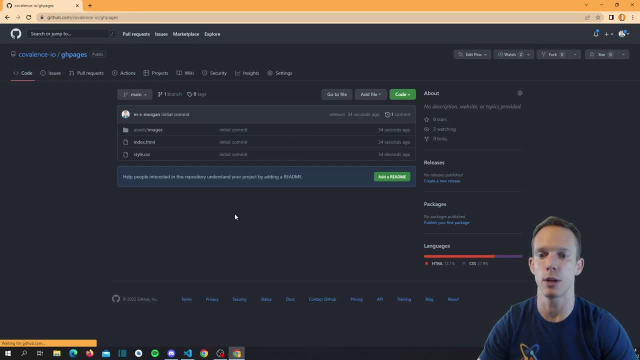 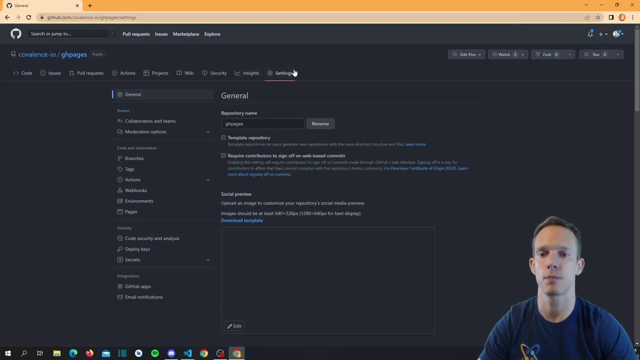 everything to main, we go back and we refresh. we can see that we actually have files in here. now we're indexed at html, we are styled at css, we have our asset images and in here we've already got aALZ Hen sane advance. so, as you can see, this thing, uh is putting in all of our devices here really quickly, but 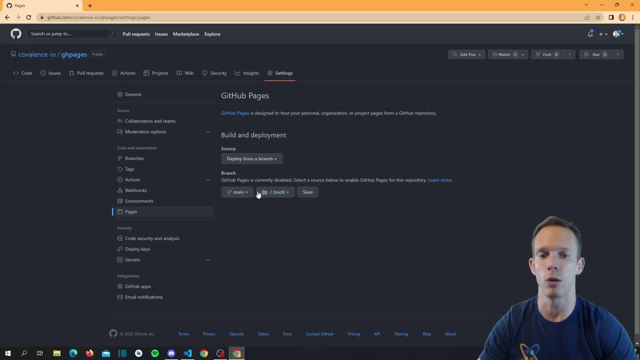 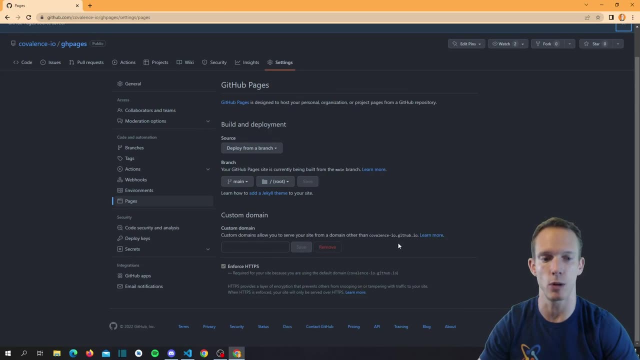 you know ap whales, and, and, and and andort founder root. all right, so we're going to go ahead and save this, and it looks like you can actually add a custom domain as well, but from right now it serves from our site domain, which is covalence. 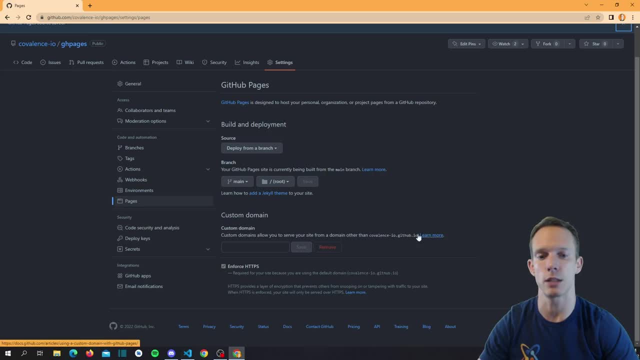 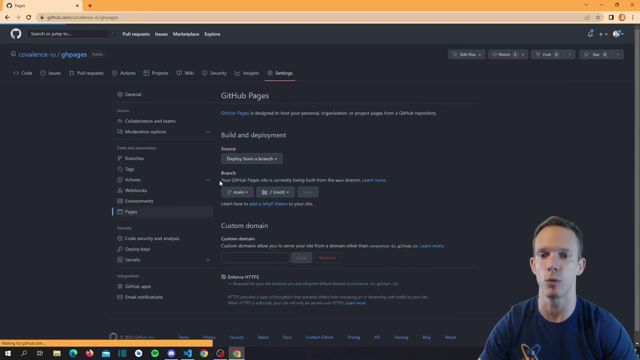 dash iogithubio, and we have https enforce, which is nice. if you didn't do that, i believe you can unenforce that if you put your own custom domain, but we're not going to be doing that right now, and so what we are going to be looking at is we're just kind of waiting for it to deploy right now. 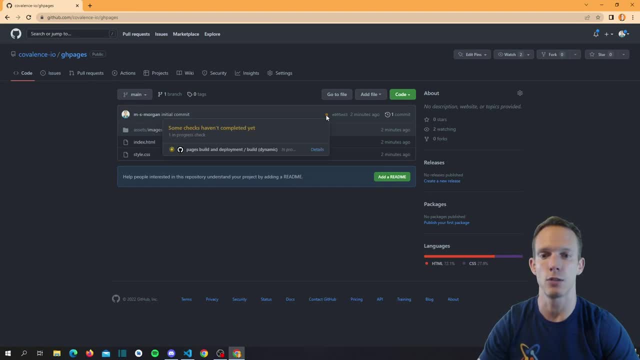 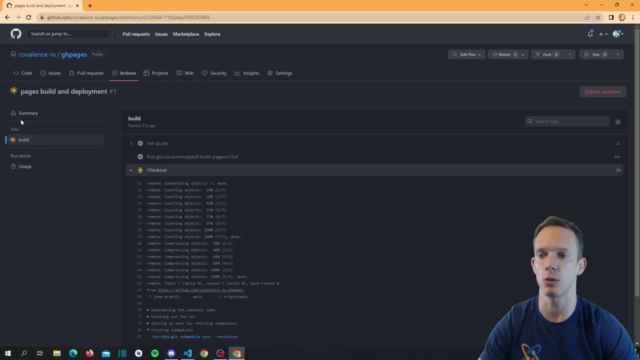 and so if you go into here you see this little orange dot. so you click that. it says some checks haven't completed yet and it actually has pages build and deployment so we can actually go into this process real quick and we can see that we have some jobs here. jekyll's doing all this fun. 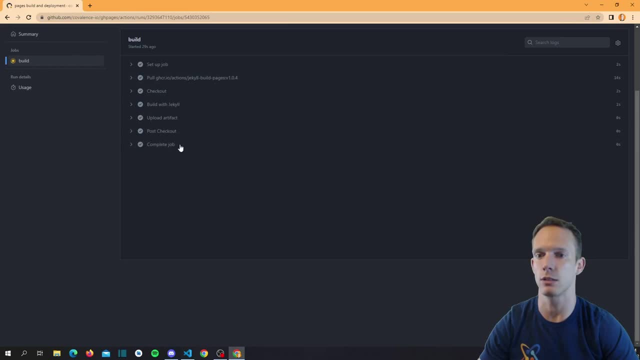 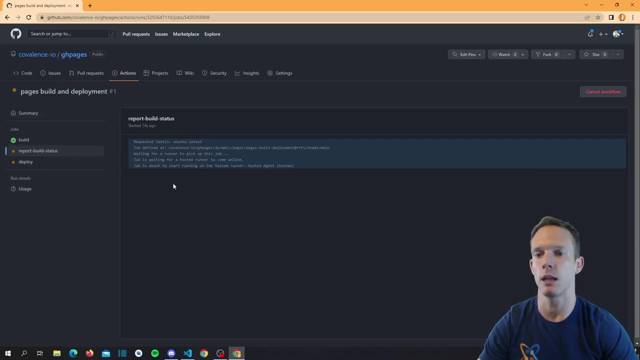 stuff, it's uploading artifacts, it's checking that this is, you know, an okay thing to actually build, and then we have our report build, and then we have our report build, and then we have our report build status here, and this is a pretty quick thing. it just actually like, does like a little report.